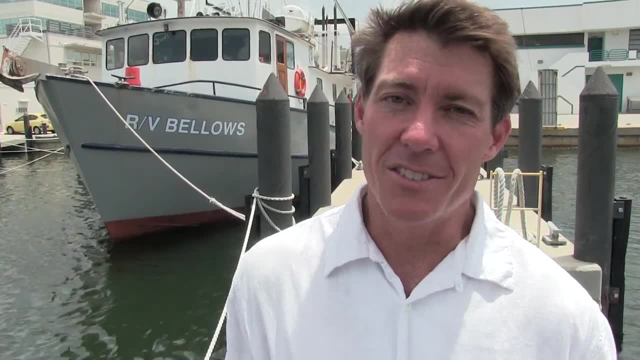 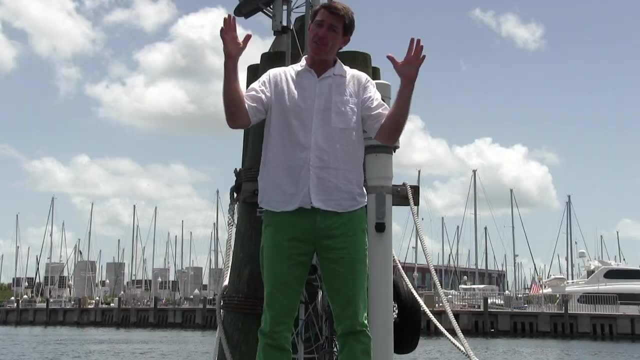 Hi, I'm Mark Hollins. When we're hungry, it's easy enough to get our fix: Just go to the refrigerator. But in the oceans, biological systems feed in a tiered paradigm. The big fish feed on smaller fish, and the smallest things are the primary producers. Those producers 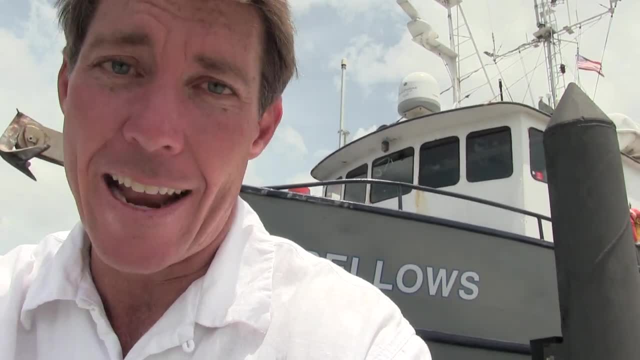 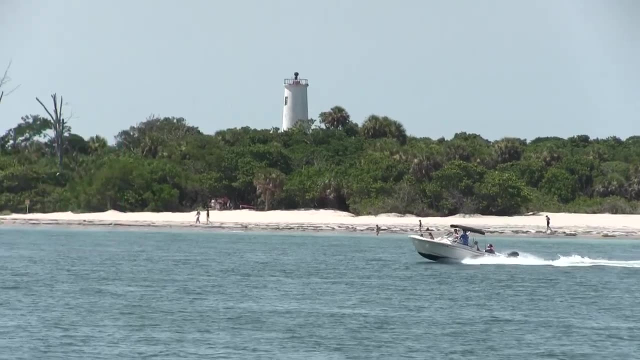 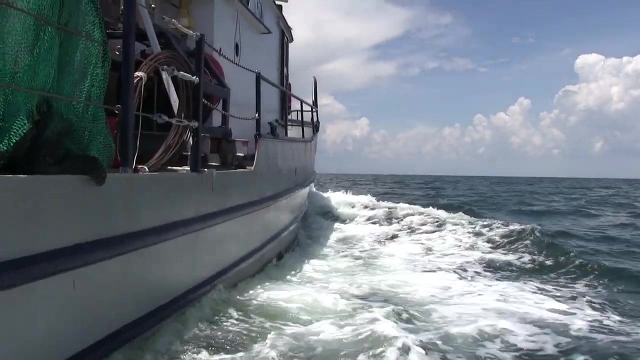 are the teeny plankton Coming up. I'm going to show you how girls look at it, with some big surprises. and take on a dare that would make most folks gag: Come aboard the RV Bellows in search of the most abundant life in the ocean, Looking out. 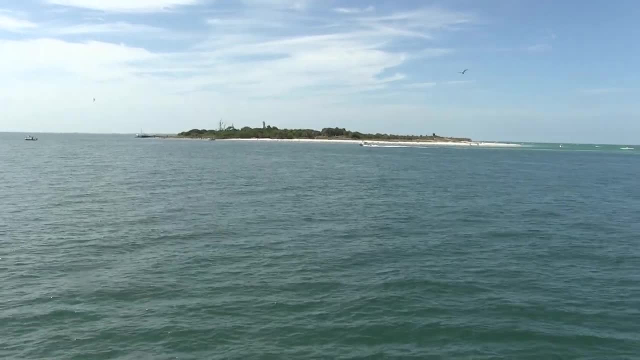 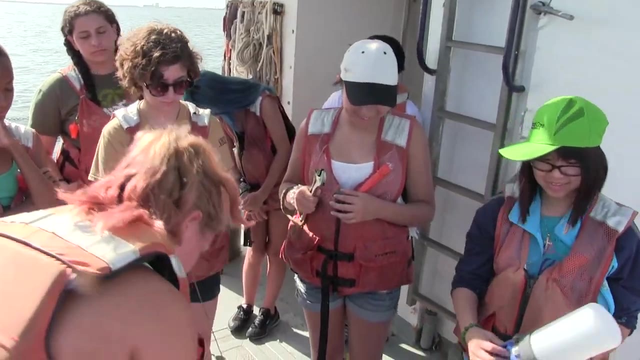 you can't see the sea drifters, but plankton is everywhere around Egmont Key. Just one drop can hold 3,000 mostly microscopic plants and animals. In this USF Oceanography Camp for Girls, 8th graders see how life starts small in the sea. Special nets are dragged. 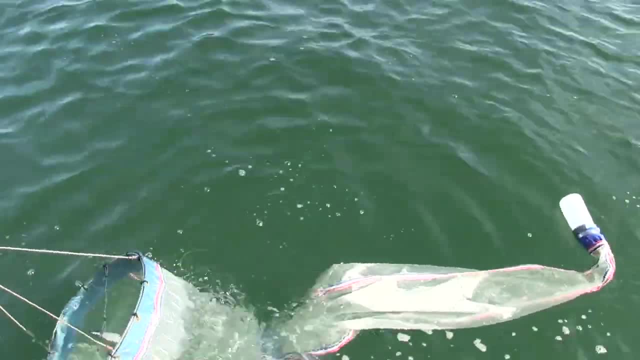 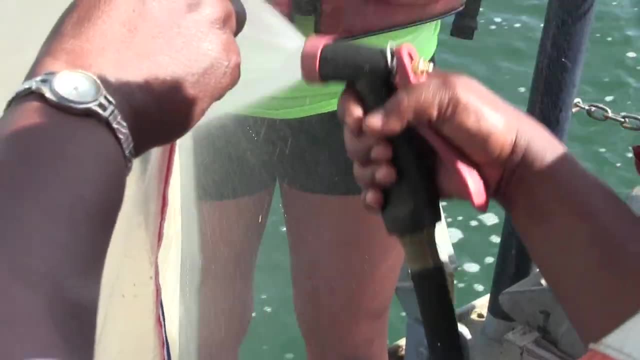 behind the Florida Institute of Oceanography's research vessel to scoop up organisms at the base of the food web. After several minutes the plankton is ready to go. Plankton nets are pulled up and hosed down with the organic briny rinse concentrated. 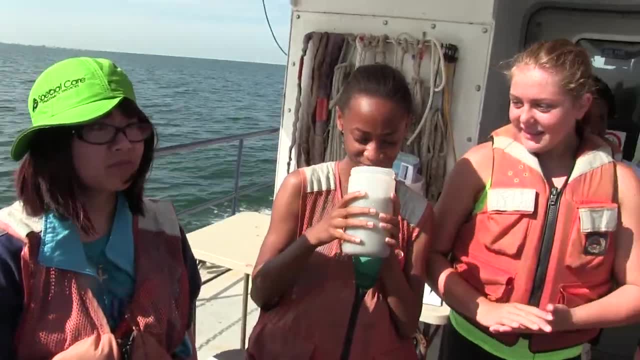 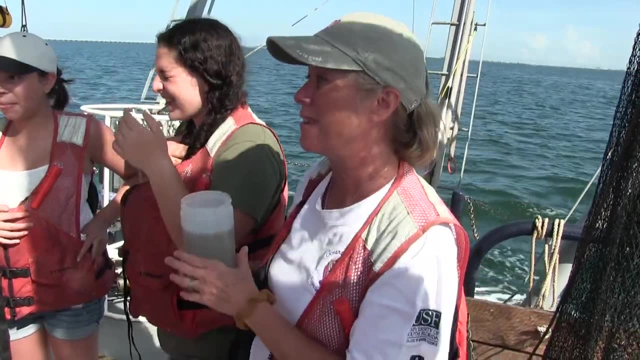 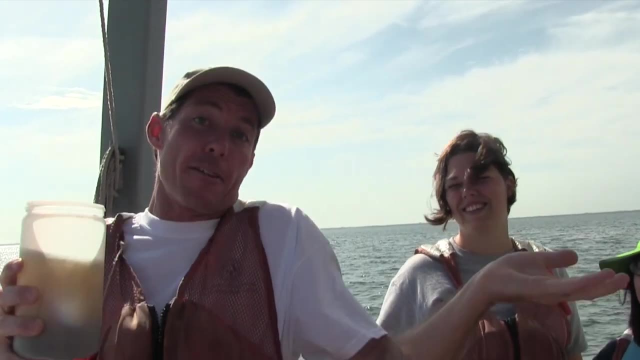 in a container. The algae stench is truly unhypotizing. Yet over the years Dr Theresa Greeley developed a learning ritual that takes courage, And I get to test the waters. Part of the study here is to look at the plankton to see the texture, to see how much length. 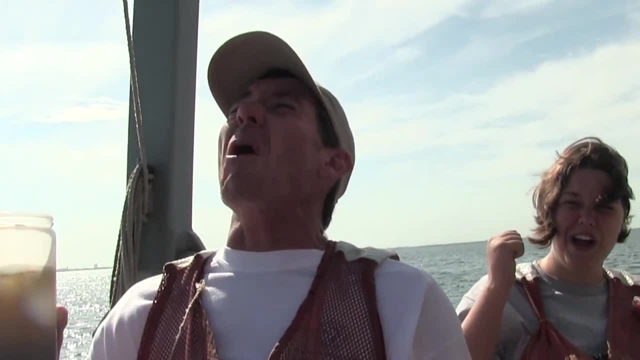 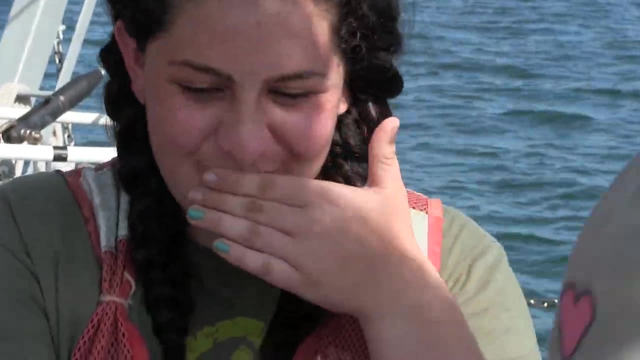 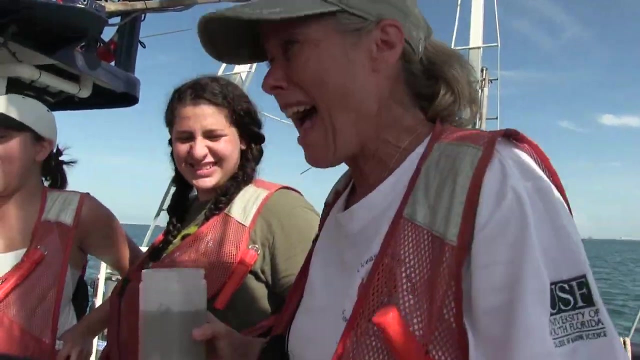 is in the cup and of course bottoms up to take it Swollen hole of sea called phytoplankton. One gulp at a time. Zooplankton- The animals that eat the phytoplankton plants. Down the hatch they go Now. had the students come face. 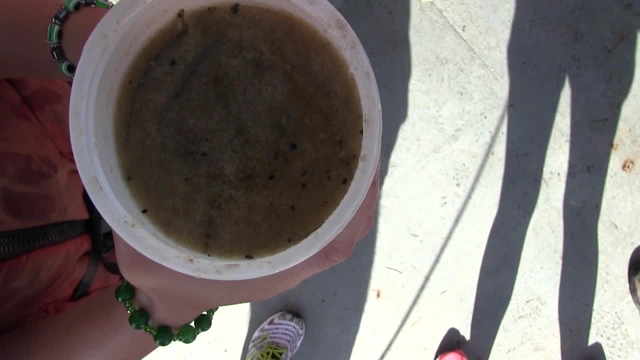 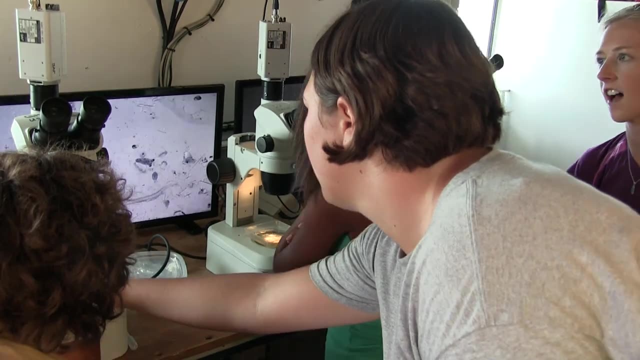 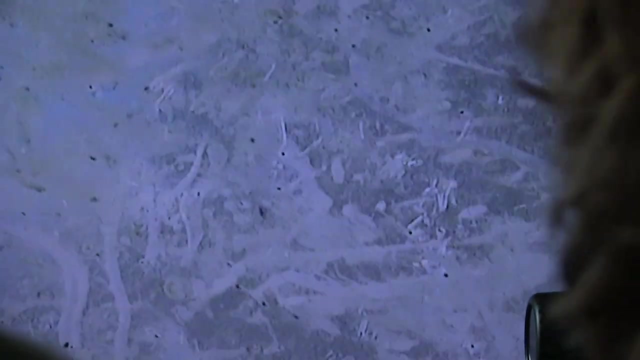 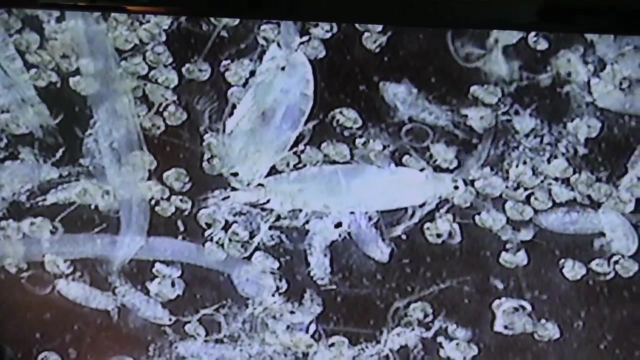 to face with the life in the cup. there would almost certainly be no takers for this communal drink. In the lab, we see a place measured by microns and millimeters and the ingredients become clear. The microscope brings the hidden into focus, revealing alien-like creatures, The armor of a copepod. 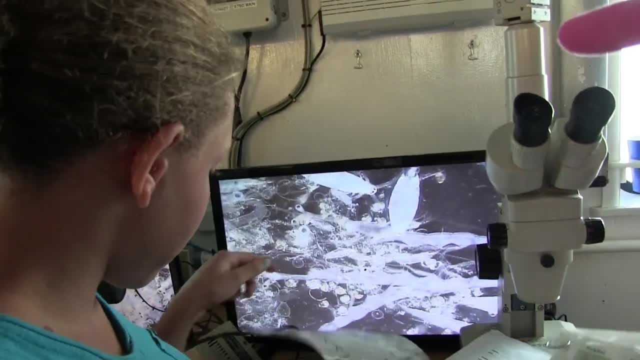 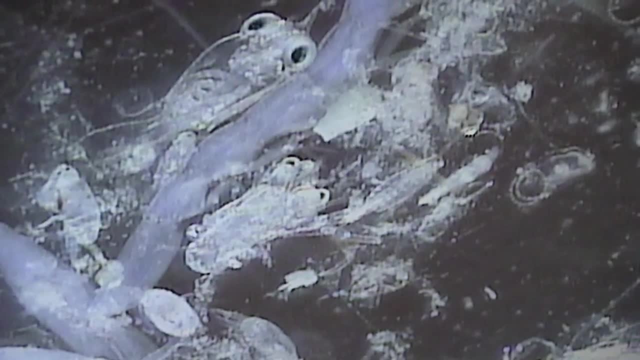 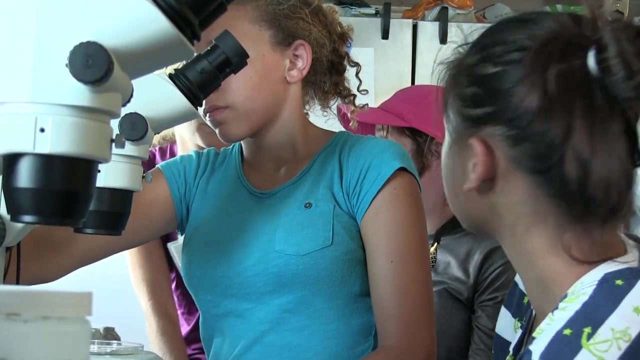 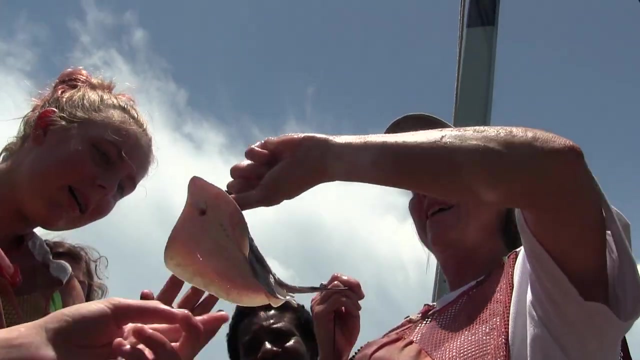 exoskeleton bumps against oval fish eggs. Diatoms intrigue students when they learn half of all the phytoplankton come from these silica based algae. Researchers spend a lifetime studying these environmental markers and learning about their miniature world to make ours better. FIO subsidized ship time encourages young women to understand marine. 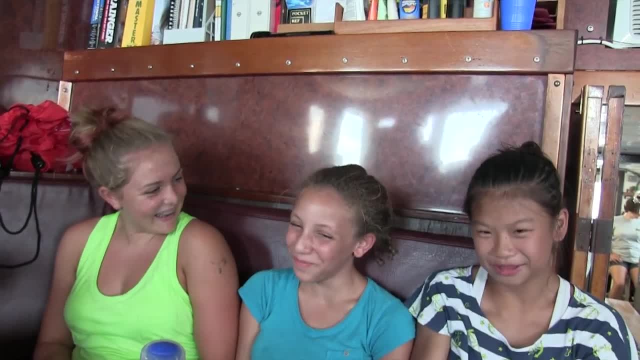 systems. Moments like these last a lifetime and promote future career interest in science. 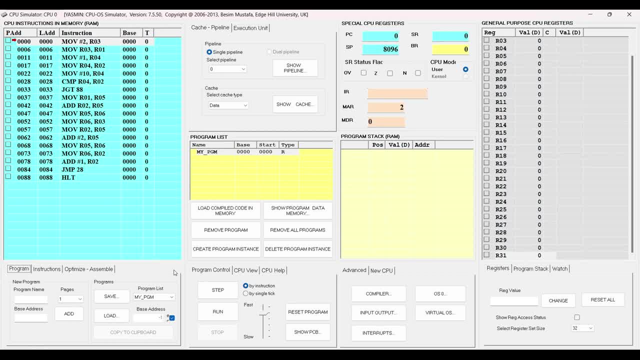 Hey there, in this video we will look into the simulation of first term first sub algorithm, also known as SCSS scheduling algorithm. SCSS, as name itself tells, serves the process which arrives to the ready queue first, irrespective of any of its priority. So now I have loaded a program in the 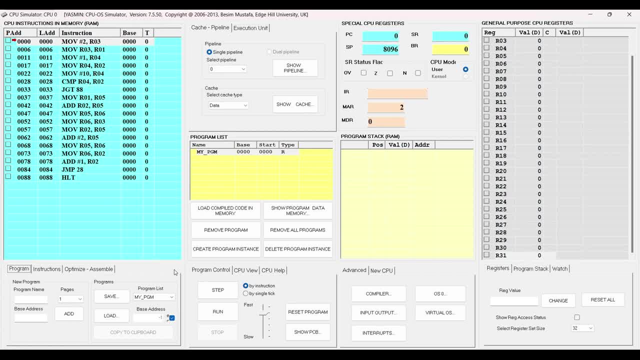 memory. and if you want to know how to load a program, you can check the link in the description or you can click on the i button on top. Also the program which I am using now. I will leave that in the description box. Now let us go to the OS options. Here we see the running queue, basically. 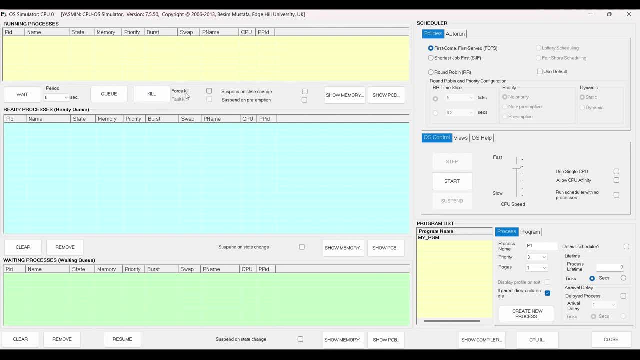 which means the process which is currently being served by the CPU is there, So we can get all those details here. After that we have the ready queue and the waiting queue. After this we have the scheduler, which has few options here. So first is the policies, which basically 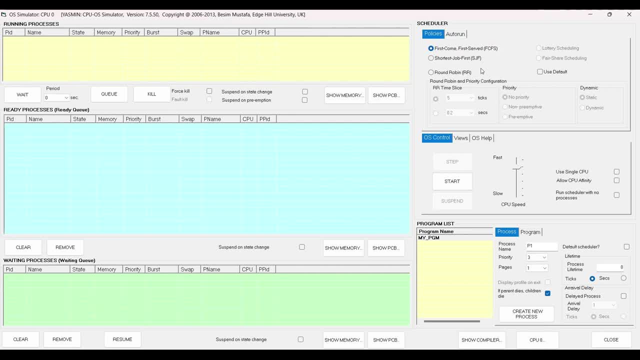 has all the policies, which namely are FCFS, strategy of first round robin and other configurations related to that. After that we have the OS control, some use and OS help. So the OS control will basically help us to start, stop the program or to increase the CPU speed. 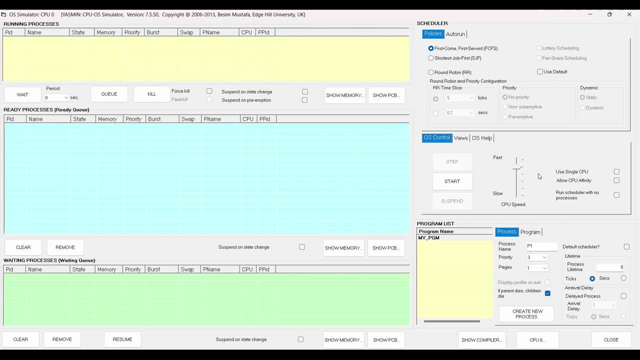 decrease the CPU speed or also some other configurations which are presented. And finally we have program list. The program list has basically the list of all the programs which we have loaded into the memory, the processes and the program. So now mainly what we will be dealing is.